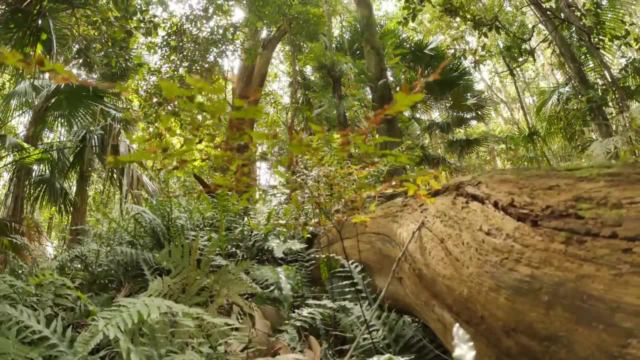 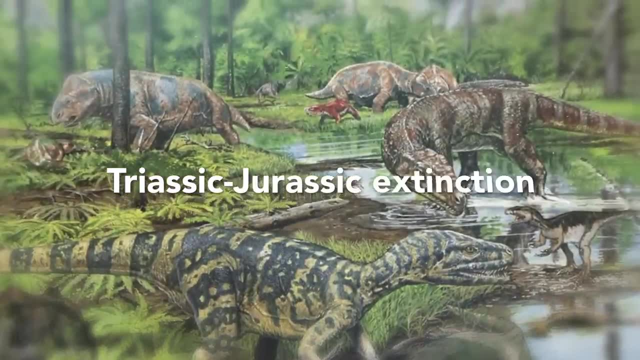 This one's going to be a bit arduous, arbitrary, but we're going to aim for between 190 million years to 230 million years ago. This was around the time of the Triassic-Jurassic extinction event, during which 20-30% of all 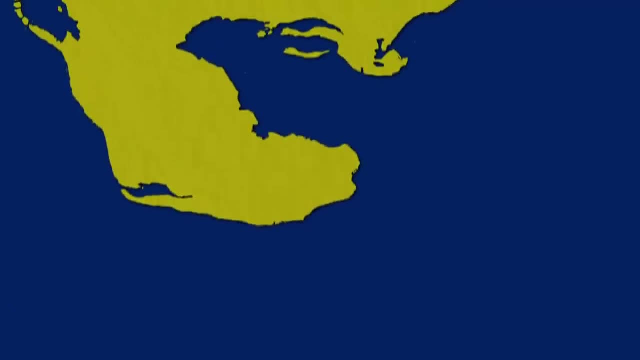 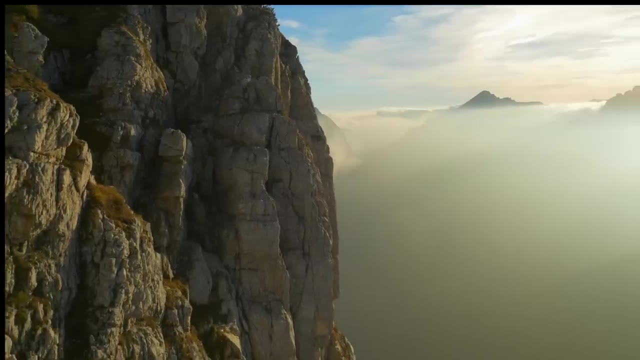 marine species went extinct. For this time, the most accurate map for Pangea I could find was this one, But using this, we can now begin to look at specific features and to start, I'd like to look at some of the mountain ranges that would and would not have existed during this. 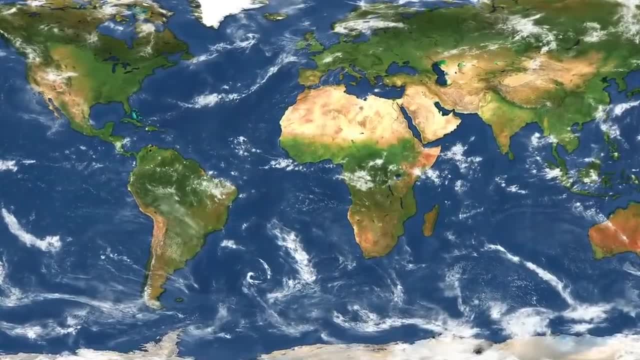 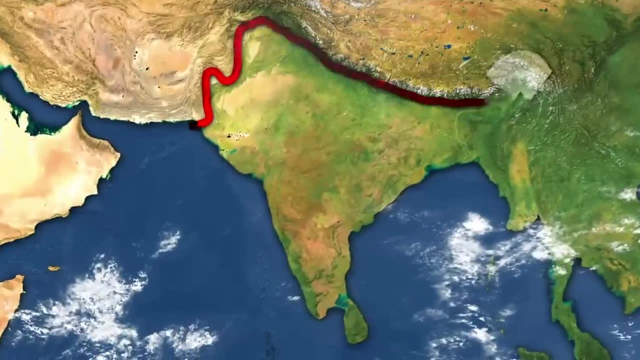 time. For starters, nearly every major mountain range on Earth today had not formed yet. The Himalayas, for example, only began to form 50 million years ago when India collided with Asia, And overall it was the tearing apart of Pangea that actually gave us many of our mountains. 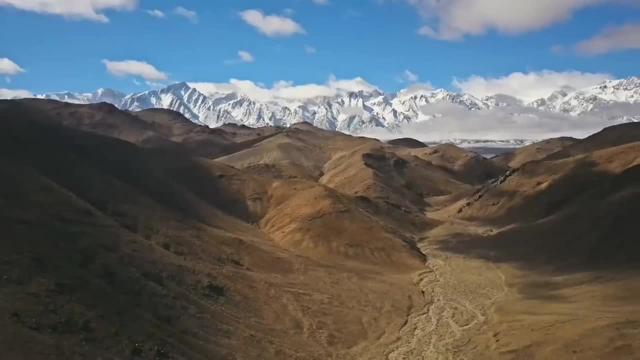 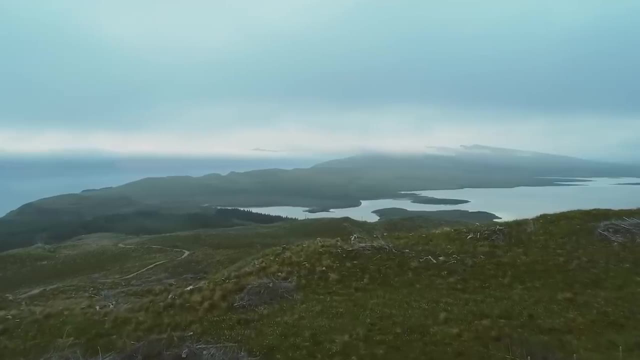 and the reason these all happen to be our tallest is because they haven't had enough time to erode. So to find out what would have been around during this time, we need to look at some of the oldest mountains remaining on the Earth, Such as the Appalachian Mountains. 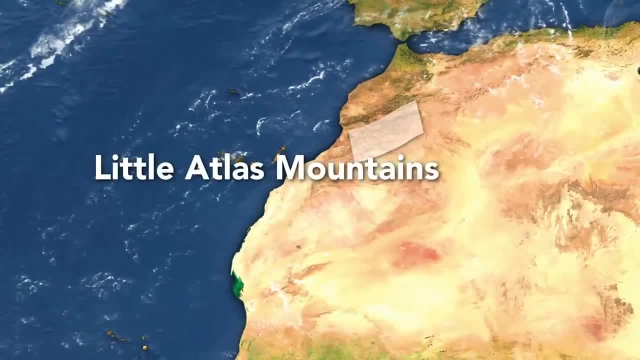 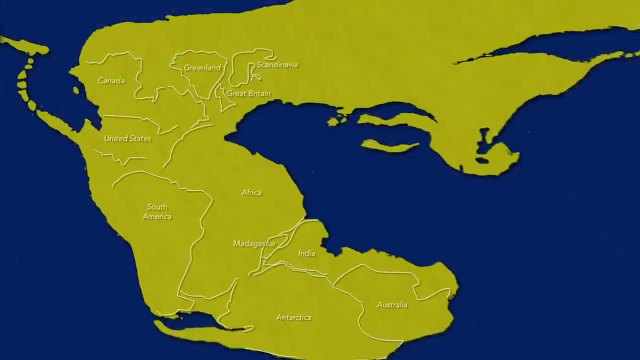 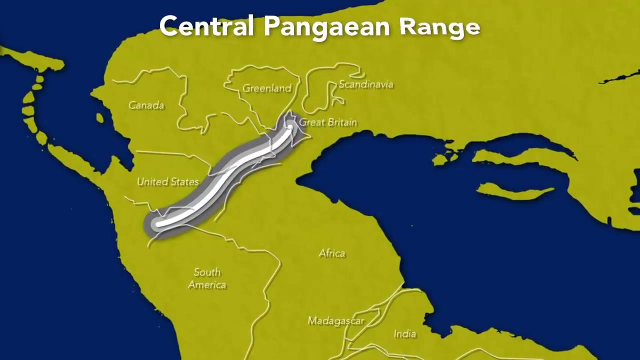 the Little Atlas Mountains of Morocco and the Scottish Highlands of Great Britain, all of which are nearly 500 million years old. Now, it just so happens that these three mountain ranges would have formed a single continuous mountain range across the supercontinent called the Central Pangean Range. 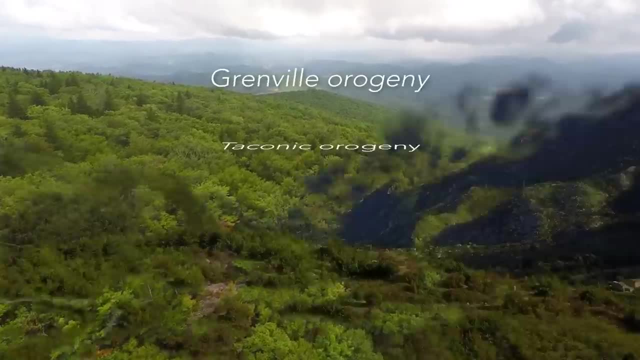 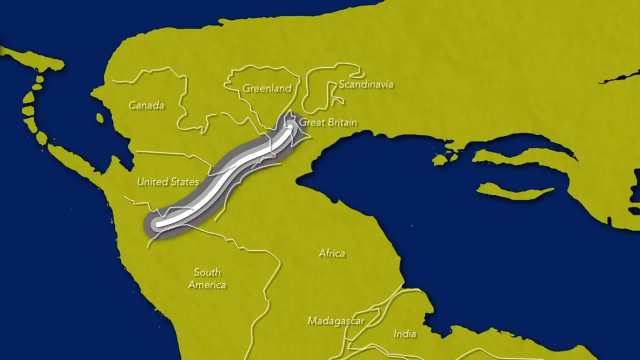 And while none of these ranges stand particularly high today, four different mountain building events in the past produced a mountain range that was once as tall as the Himalayas are now Essentially separating the continent between the two remnants of older supercontinents, Gondwana and Laurasia. 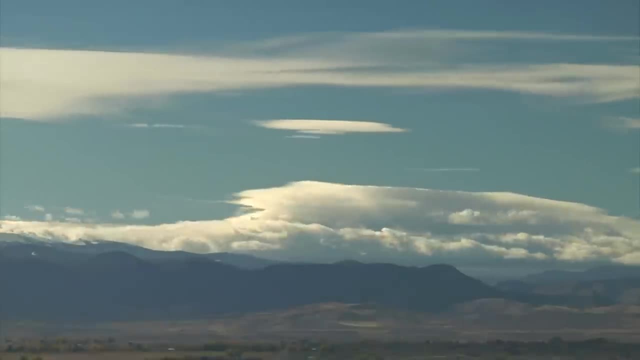 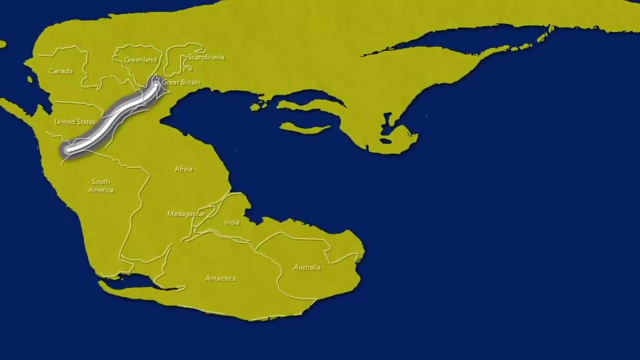 It was only with several hundred million years of weathering and erosion that these once great mountains were whittled away to the gentle slopes of today. However, there were, of course, other mountain ranges here as well. Nearby the Laurentian Mountains of Quebec, reaching into Greenland, for example, were 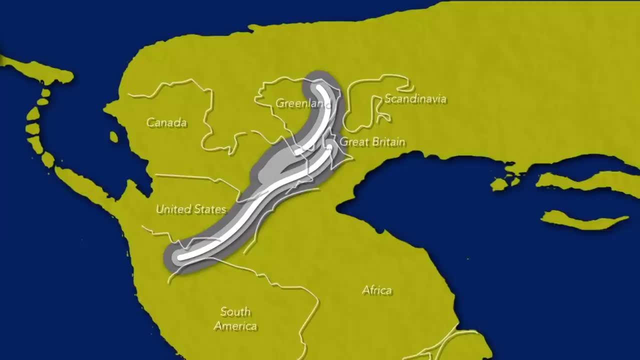 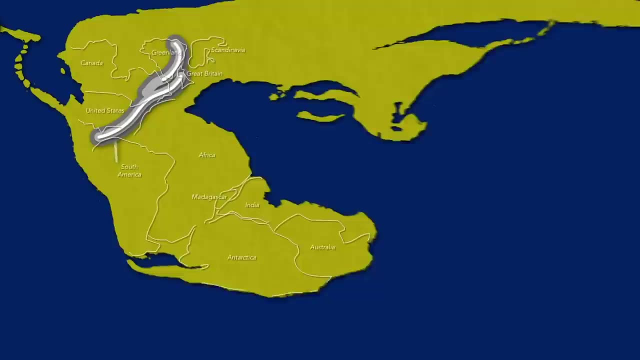 also created during the Grenville Orogeny, making this area of Pangea, occupied now by Canada and the United States, Some of the most mountainous land on the earth at the time. Then there was the Guyana Shield, a series of mountains and highlands in South America. 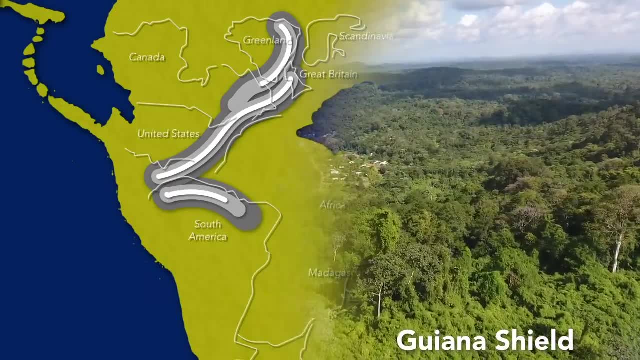 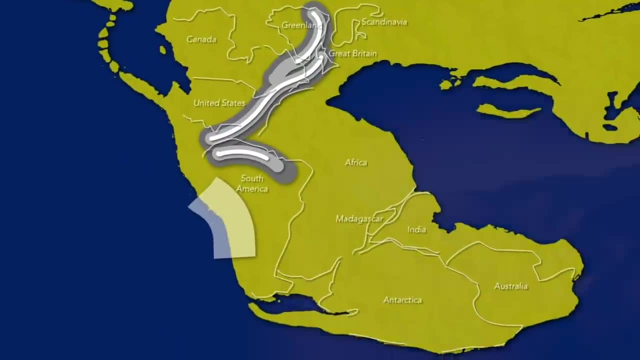 with a history that extends back nearly 1.7 billion years, though you can just barely make it out on modern elevation maps of the region. We also would have seen some of the earliest mountain building in the Andes, with the start of the Andean Orogeny. 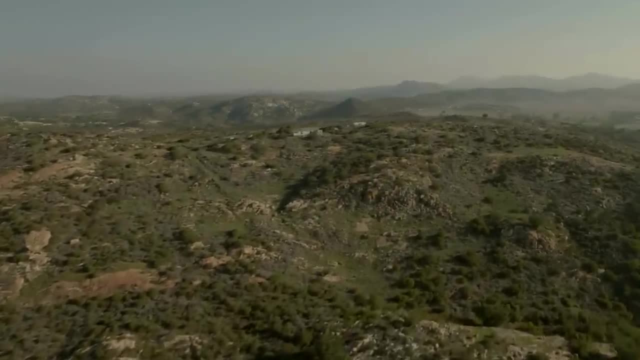 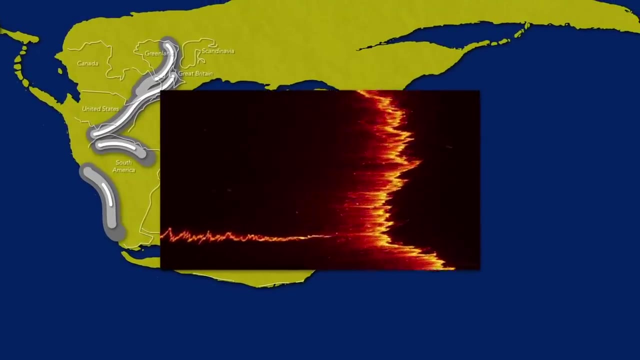 These would have been just the beginnings of mountains, however, and nothing like what they are now. Then, as the lower section of Pangea- What was previously Gondwana- began to tear itself apart, splitting Africa from South America, Mountains were created around the divide, resulting in the mountains of Eastern Brazil. 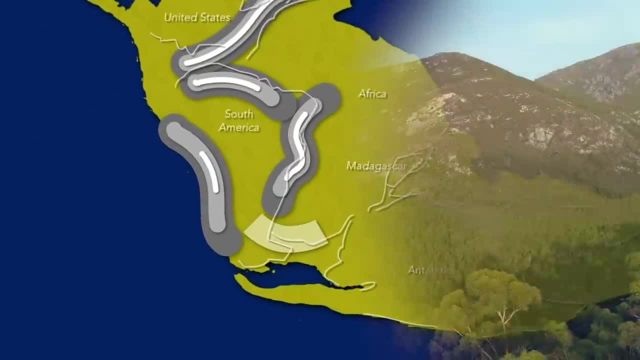 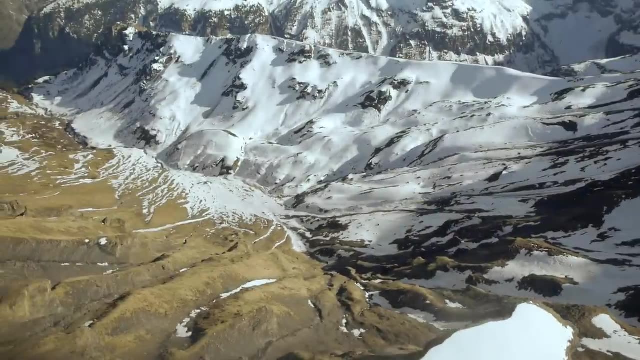 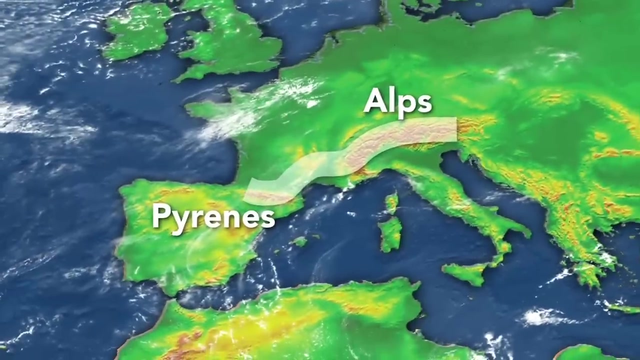 and Western Africa. South Africa is actually where many of the world's oldest mountain ranges are today, with the oldest being the Maconjua Mountains. Lastly, I want to talk about the Verscan Orogeny, which was another substantial mountain building event that led to the growth of the Alps and the Pyrenees in Europe and spread all the way. 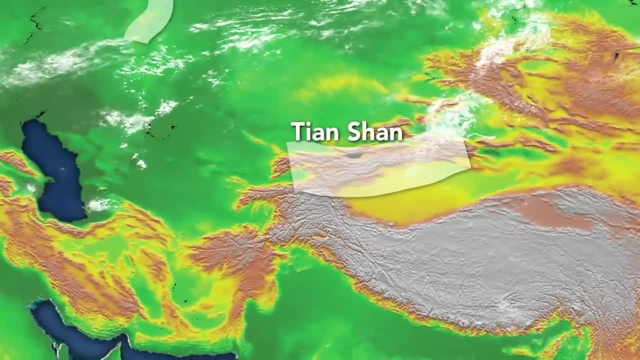 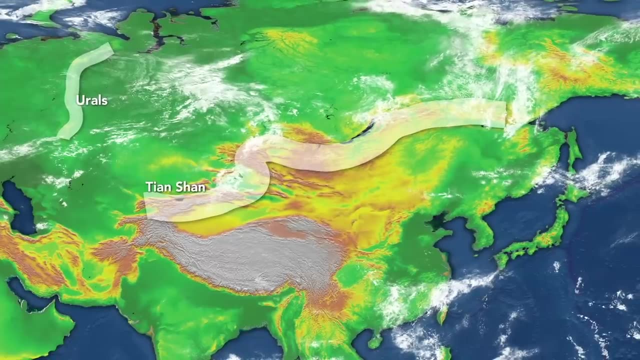 out to the Ural Mountains. This is where the mountains of Russia and the Tian Shan Mountains of Central Asia, as well as many other mountain ranges sprawling all the way to the far coastal Primordia region, also in modern day Russia. This places mountains roughly along these lines on our map of Pangea. 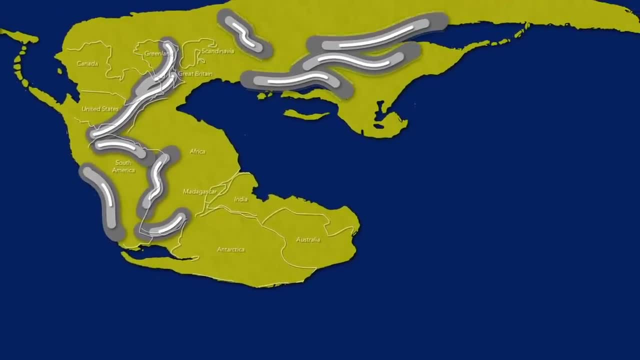 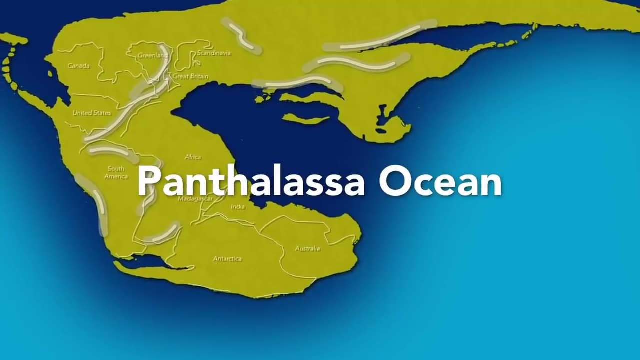 And with that we've finished making the important mountain ranges at the time. After mountains, next, I'd actually like to talk about the ocean. First, there was the Panthalassa Ocean, the ocean which encompassed most of the world, with its name literally translating into the Alps. 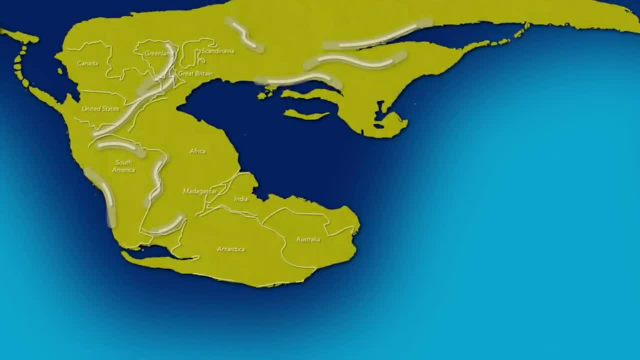 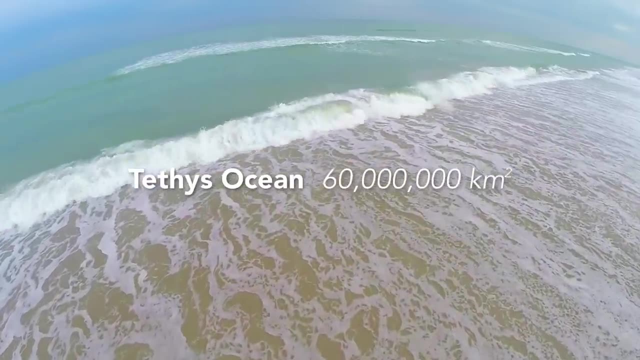 And then we'd get the beginnings of the Tethys Ocean. if considered separate from the Panthalassa Ocean, And this body of water would have been around 60 million square kilometers, a bit smaller than the Indian Ocean today, but still much larger than the Arctic Ocean. 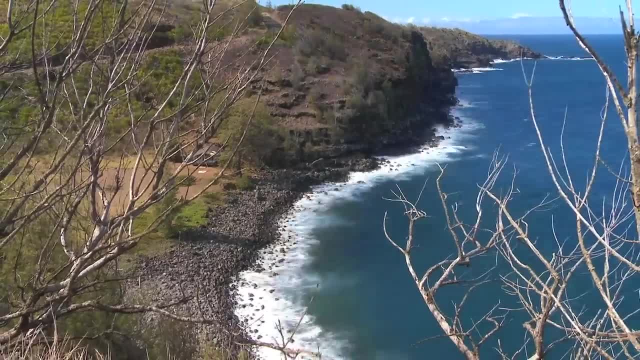 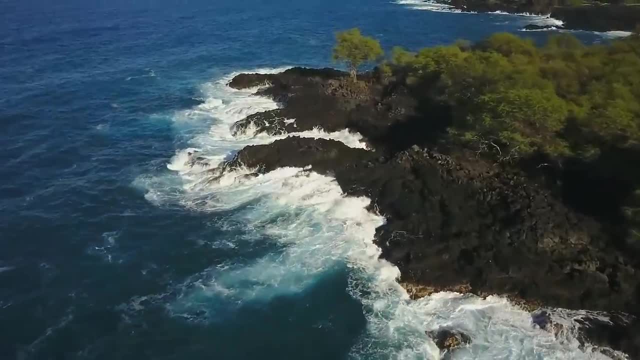 What I'm interested in, however, isn't the size of these oceans, but how the ocean during this time would have influenced the climate and ecology of the land. I don't think anyone will be surprised to hear that the ocean can affect climate in multiple different ways. 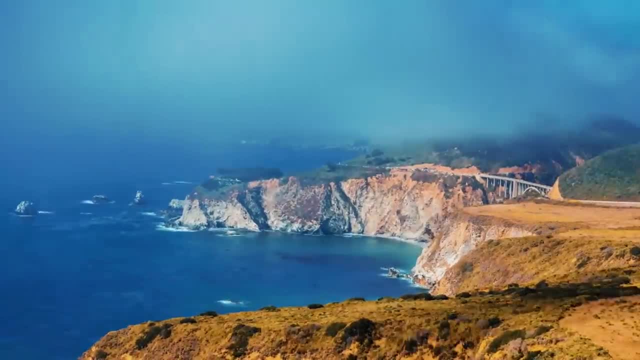 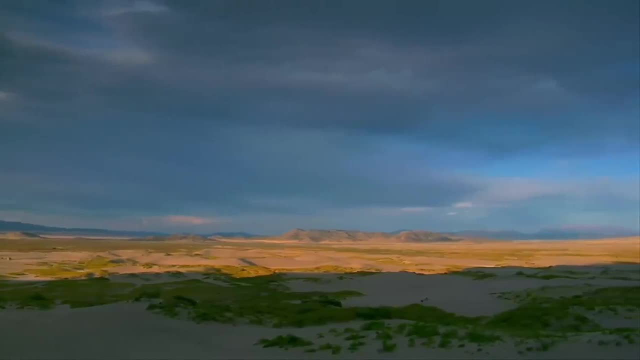 In terms of rainfall, lands directly beside the ocean will typically experience greater amounts of it, While the continental interiors- the lands furthest from the ocean- will become increasingly arid. We can see a similar effect taking place across Central Asia today, where, due to its remoteness, 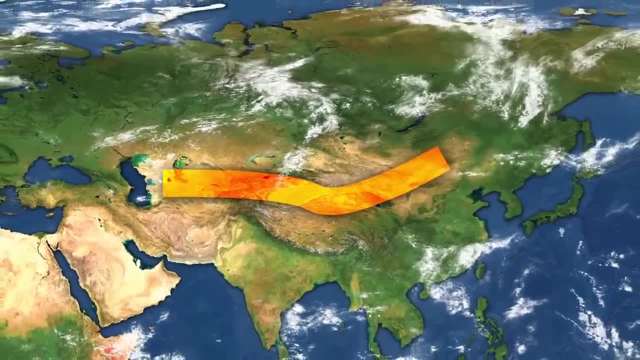 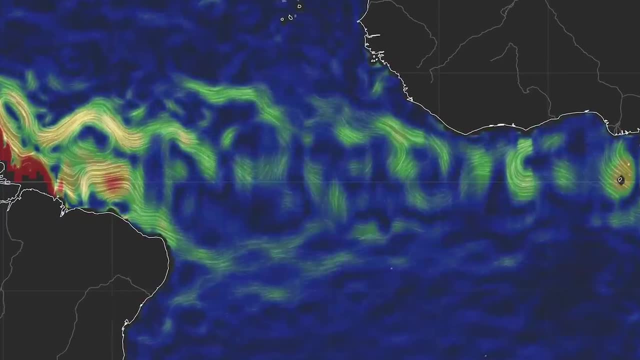 a band of dry regions can be found crossing nearly the entire body of Asia, But I wish it were that simple. The thing we really need to look at is ocean currents, or how the waters of the ocean would have circulated around the world during this time. 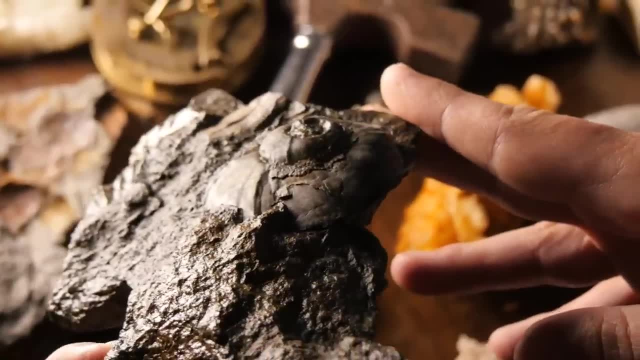 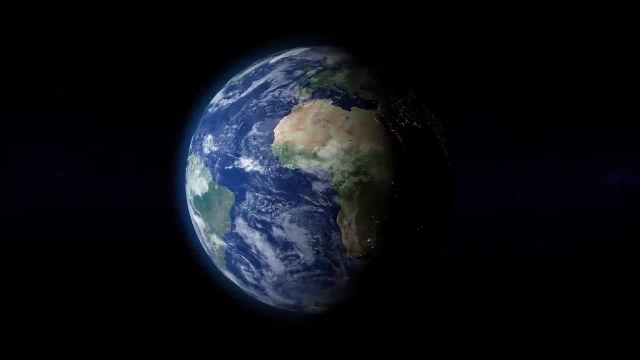 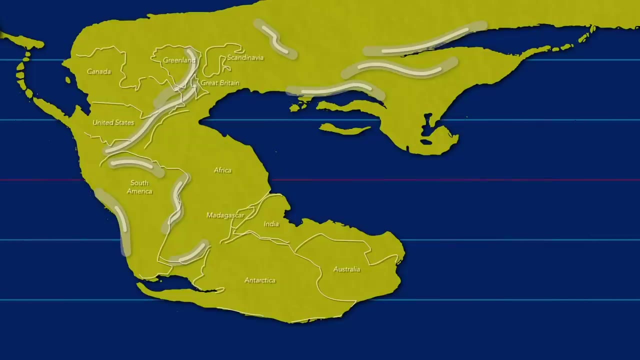 Now there isn't really great fossil evidence for what ocean currents would have been like, so there's nothing really tangible for us to go on. But we still know how the earth was rotating- basically the same way it does now- And because of this we know that the wind patterns across the earth would be virtually 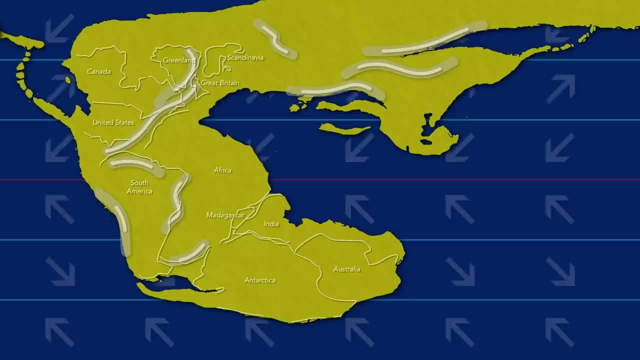 the same as they are now, meaning they'd look like this: Now it's the winds that push surface waters around, so knowing these winds, we can reconstruct a general schematic for water circulation, At least at the surface. Let's take a look. 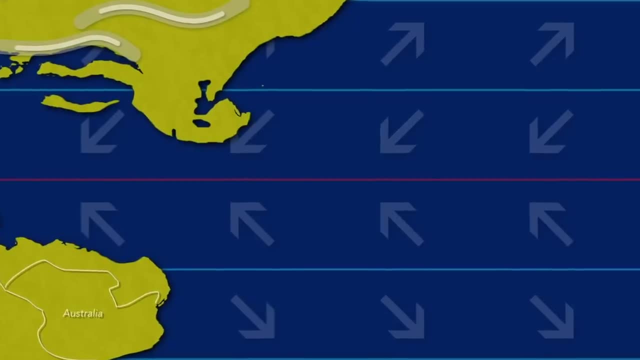 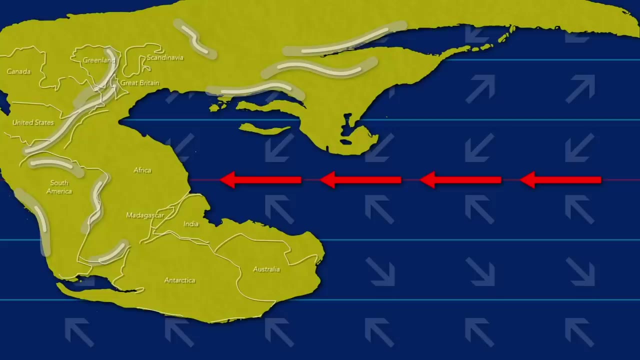 First by the equator. both winds from north and south push the water in a westerly direction, creating an ocean current moving to the west across equatorial waters. Because it's at the equator, these waters will also be warm water currents, which will 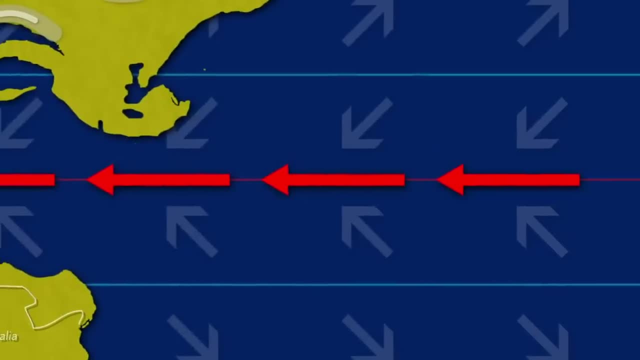 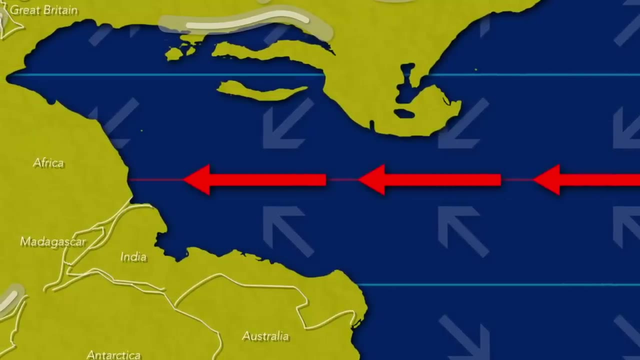 be important later. This equatorial current would continue flowing westward from the panthalassa ocean, pushing warm water into the tethys, until it reached land. Where this happened, the waters would have been diverted around. In the northern hemisphere, this sends water upwards. 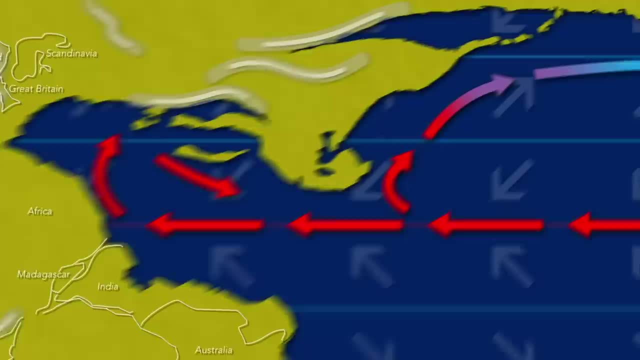 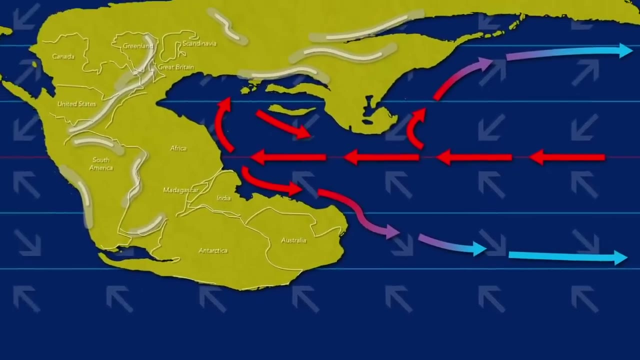 And eventually back out cooling down in the process In the south, well, a similar thing happens, as the water deflects and cools down a little before getting sent back east, Tracing these water movements onto the other side of the continent. we'd still have that. 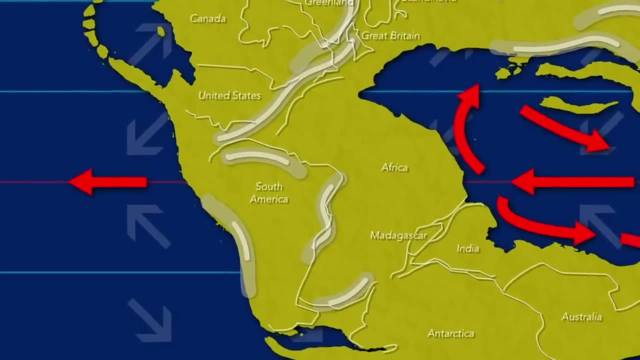 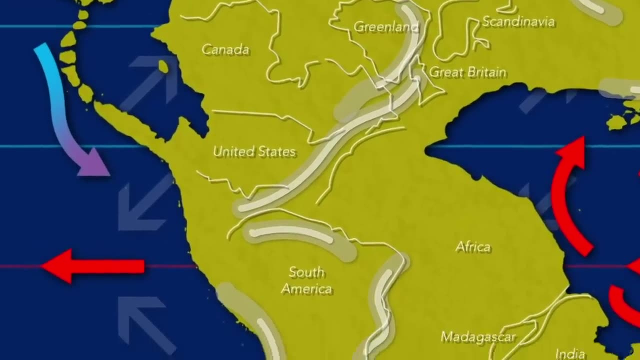 westward moving current at the equator. due to the trade winds In the north, this current would have mostly deflected downward, with some of it straying into this northern inland ocean area. The downward flowing waters would begin warming back up, eventually joining the equatorial. 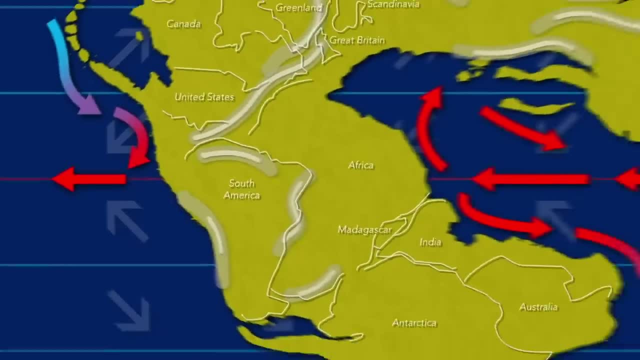 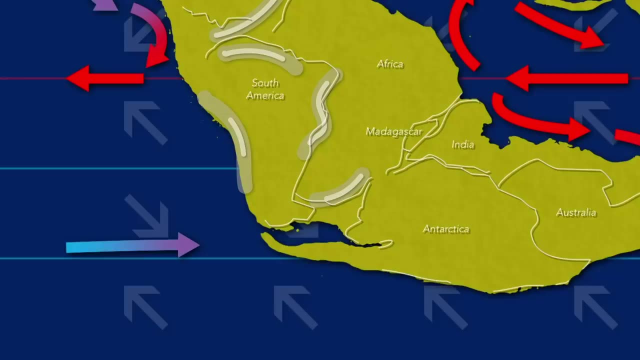 current completing the northern ocean giant. In the south, the current would have to travel a bit further until it came into contact with this shoulder of land. Here the waters would divert around as well, with some of them traveling back up north. 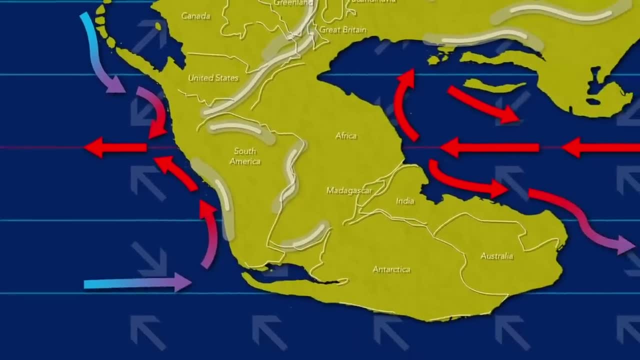 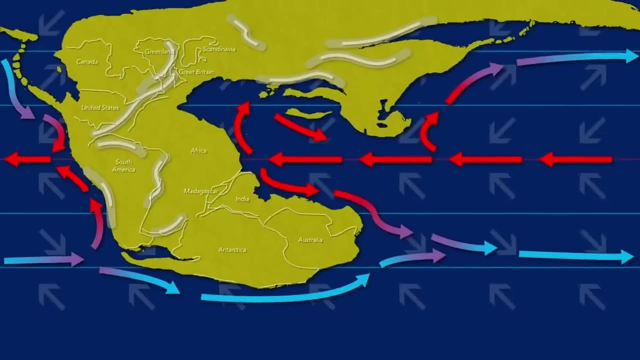 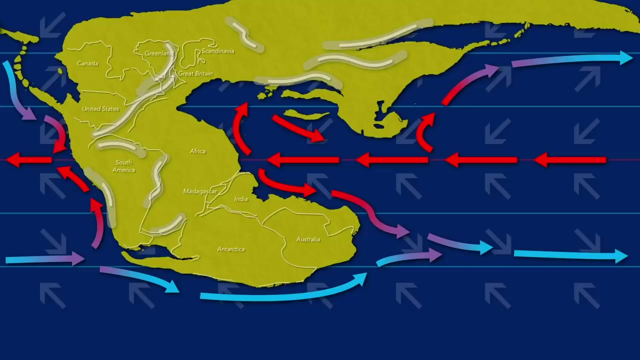 again warming in the process, And then some of the water would also divert to the south and travel as cold water across the southern end of Pangea until joining with the currents here and keeping on eastward, completing the southern ocean giant. And there you have it: a basic illustration of what the ocean currents that interacted. 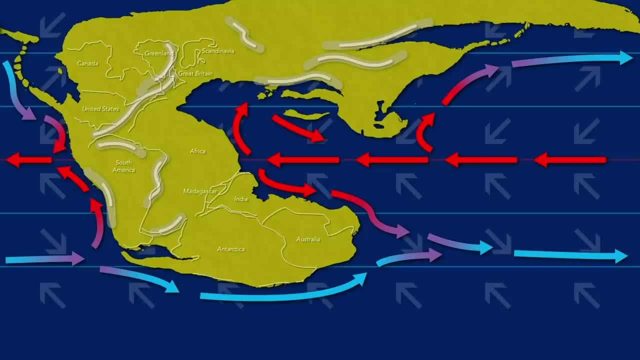 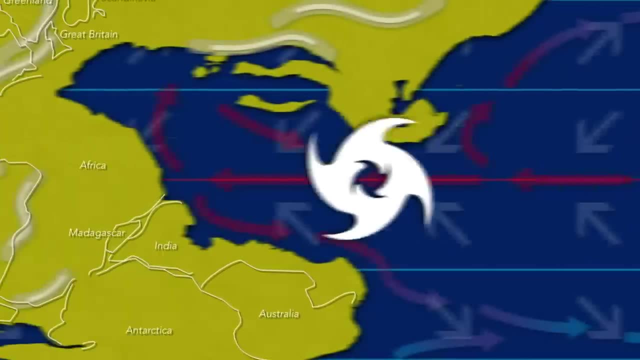 with the lands could have looked like. Lastly, and I'm not going to really explain why, there would have been a yearly equatorial monsoon season blowing great amounts of rain from the panthalassa into the tethys, inundating many of the lands surrounding the tethys ocean with great amounts of water. 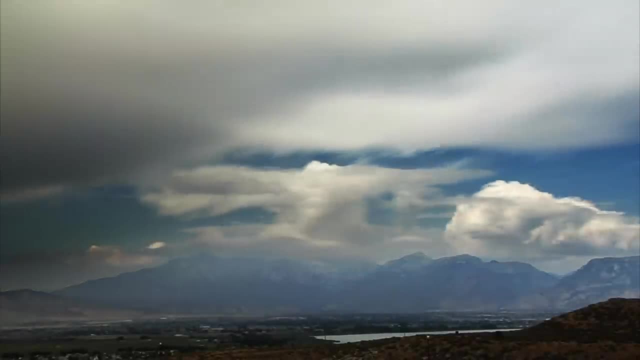 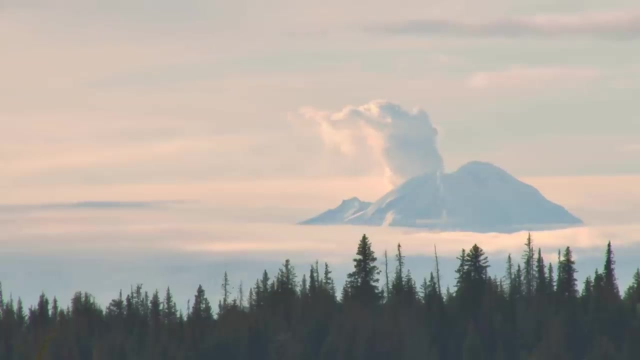 Knowing these simple characteristics about the earth and its ocean at this time, we're almost ready to start figuring out the land cover. But before we do that, we need to know how different the conditions of the earth would have been compared to what they are now. 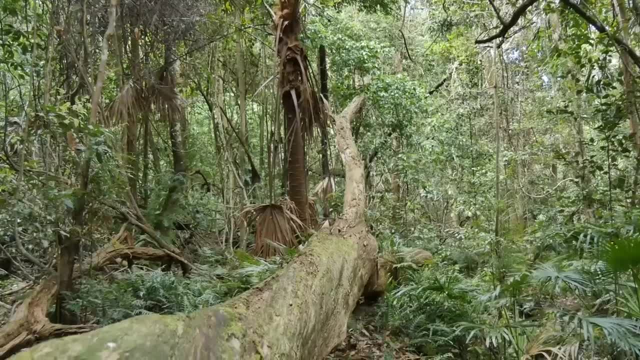 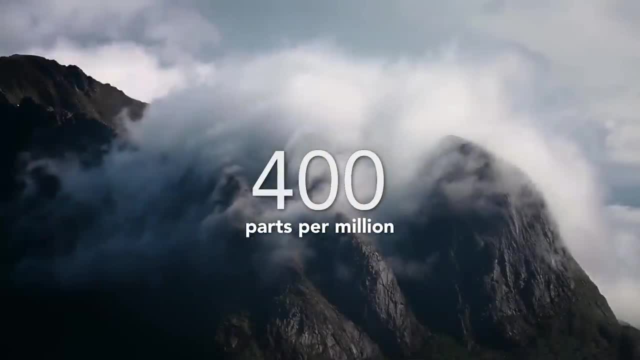 1. CO2 Concentration. 200 million years ago, average carbon dioxide levels would have been around 1,850 parts per million in the atmosphere, compared to 400 parts per million we're hovering at today, Meaning the CO2 concentrations around this time would have been about 5 times greater. 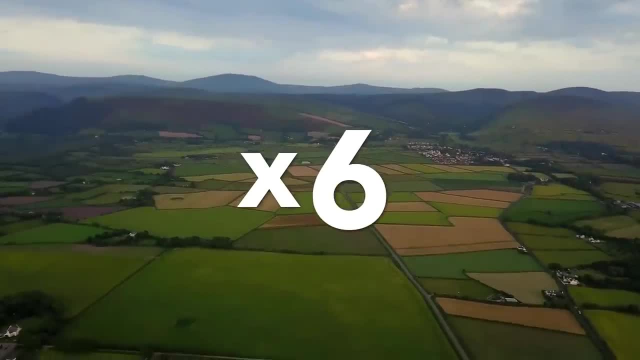 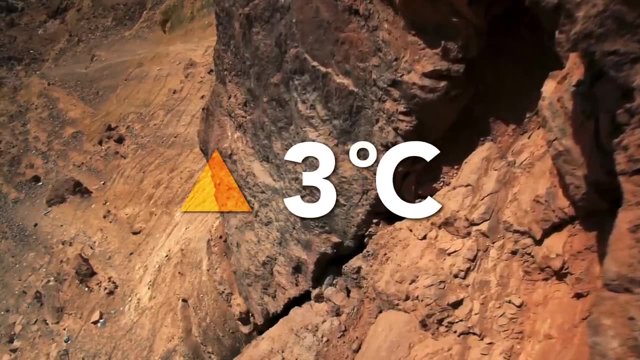 than what it is today and 6 times greater than what it was before the industrial revolution. This would have resulted in global temperatures averaging roughly 3 degrees celsius warmer than modern times, And while this might not sound like a lot, But it's not. 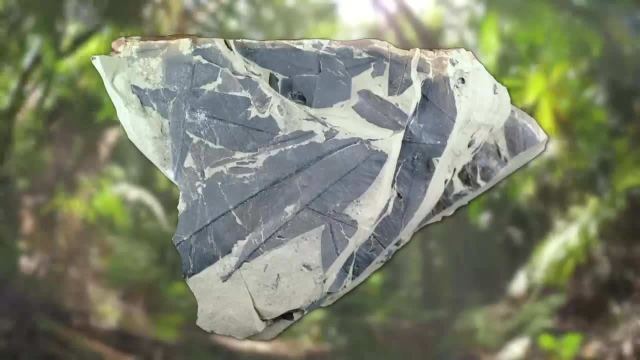 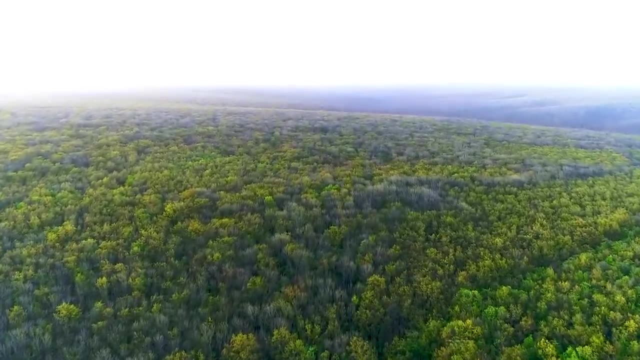 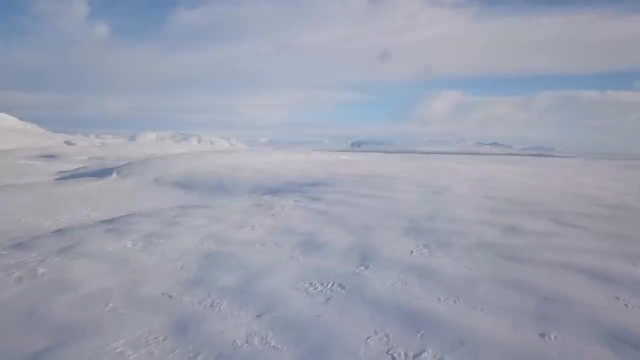 The results from the north pole 200 million years ago show subtropical and even some tropical plants growing here, and there's absolutely no evidence of glaciers or really any ice existing on earth at this time, besides maybe within the mountain ranges. In other words, this would have been a greenhouse earth where even the north pole could have. 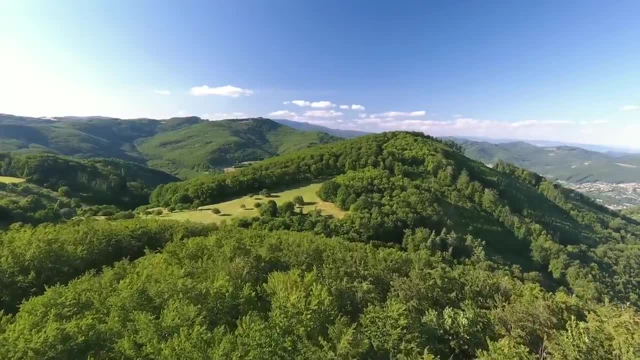 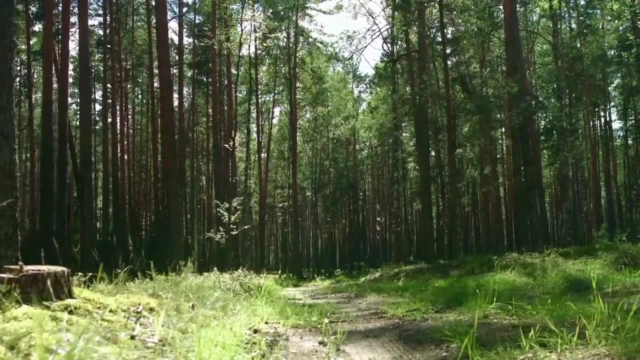 been covered in tropical rainforests if the moisture levels were right, Because only warm climate environments could have existed at this time. this rules out the existence of any large temperate environment. So if temperature was less of a deciding factor at the time, this would have made moisture. 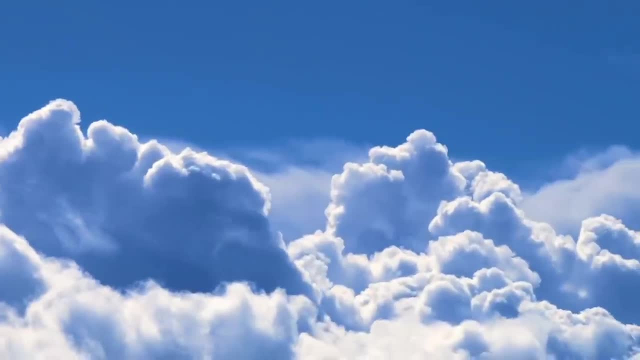 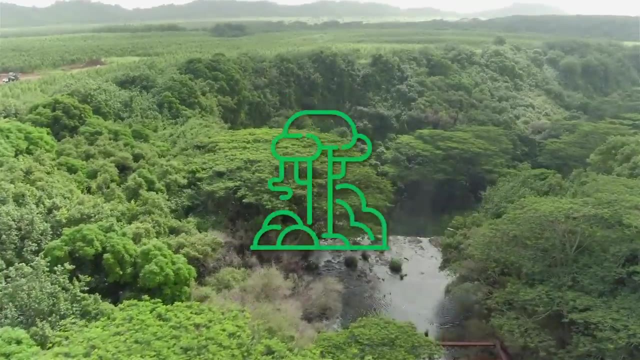 the primary determining factor for the environment. Because of this, the lands of Pangea would have been balanced between basically two radically different environments: Where it was wet, there would have been forests, and where it was dry, there would have been hot deserts. And, of course, where it rained a moderate amount, a narrow tropical savanna would have appeared as a transition zone between the two extremes. This would have been a very different environment. If we look at the ocean, currents and mountains, then we can start to figure out where there. 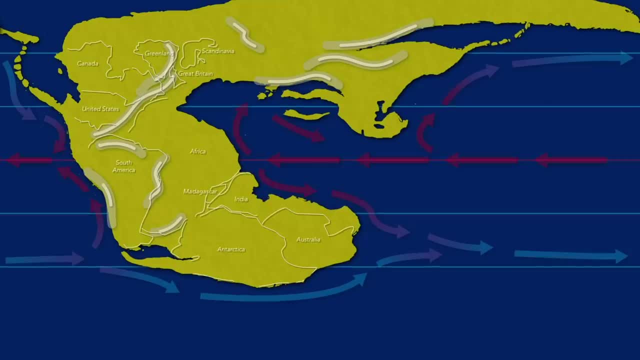 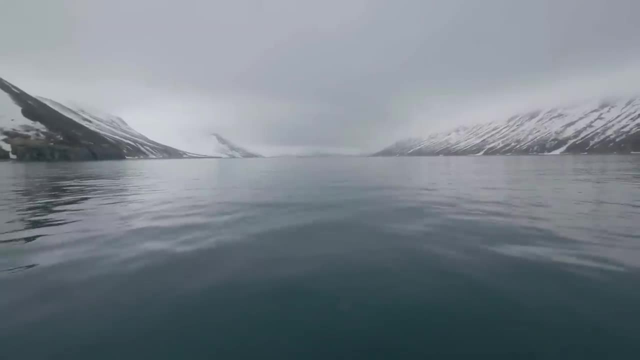 might have been forests and desert, and then fill in the lands between them. with savanna To start, I'm first going to look at the ocean currents. Cold water evaporates very little, producing very low levels of moisture in the atmosphere, which in turn produces only small amounts of rain. 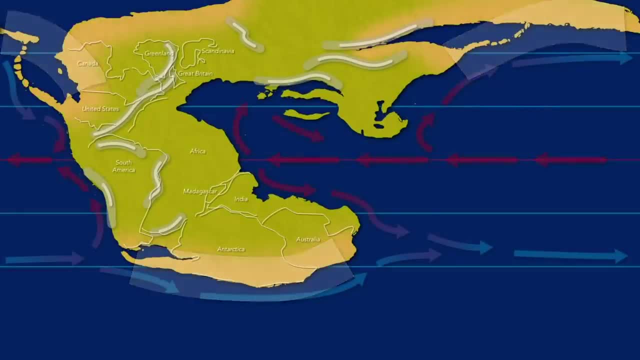 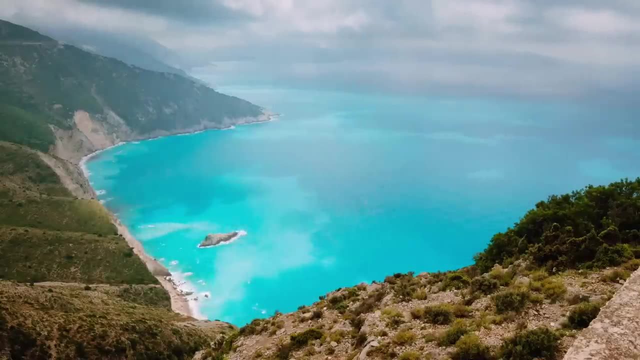 So, beside lands with cold currents running along them, I'm going to put deserts. Inversely, where the surface waters are warm, evaporation occurs more readily, filling the air with moisture Which eventually falls back to the surrounding earth as rain. 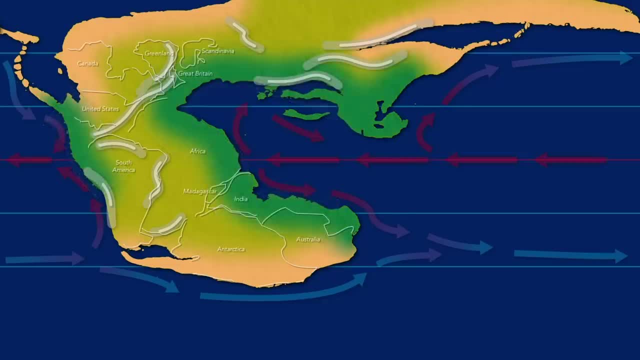 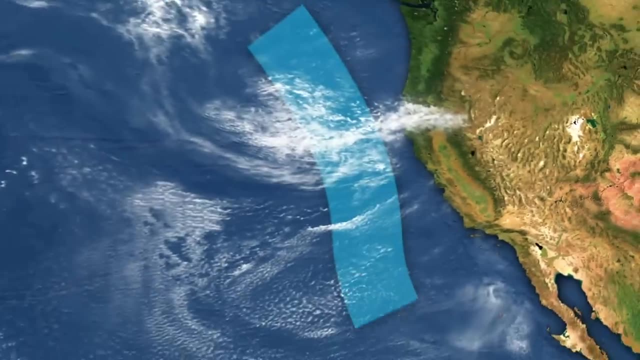 So wherever warm waters flow beside the land I'm going to make into forest, These trends still clearly exist to this day, by the way, like off the coast of California, where cold ocean water moves, turning the land here pretty arid and creating environments. 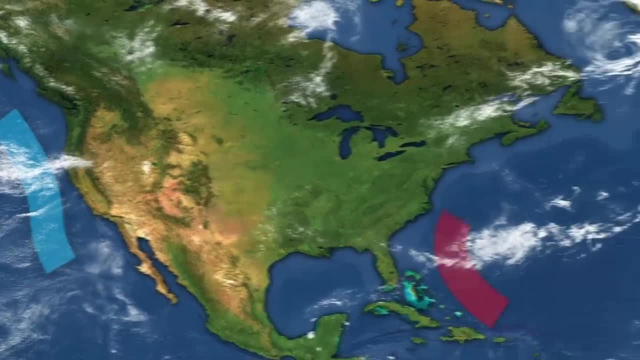 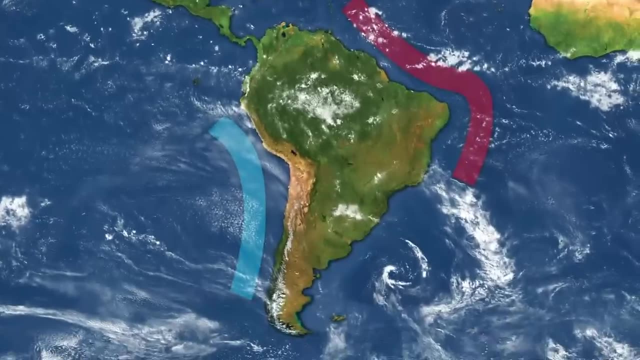 like the Mojave Desert, While on the other side of the US, warm Atlantic waters flow up from the Caribbean, resulting in a much more humid eastern United States. This is also true for South America, Africa and Australia. However, this is not the case for the rest of the world. 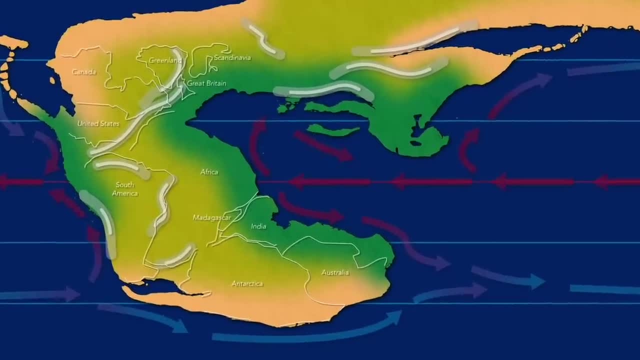 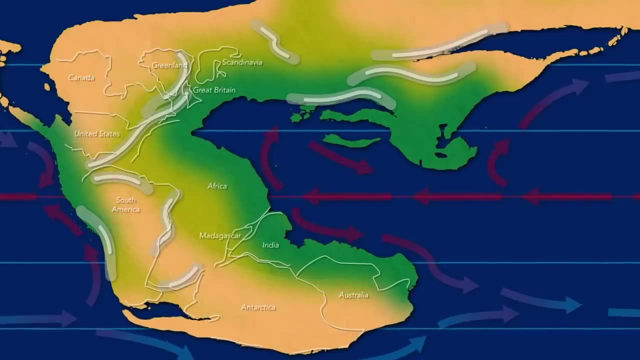 This is the case for the rest of the world. However, I mentioned earlier that the further into the interior you go, the likely the drier it would become, So I'm also going to push the deserts further into the interiors, where they already exist. 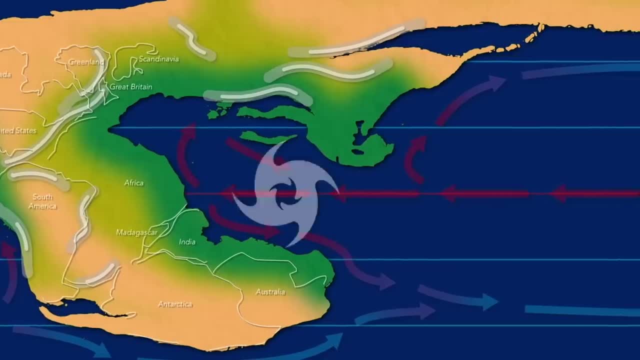 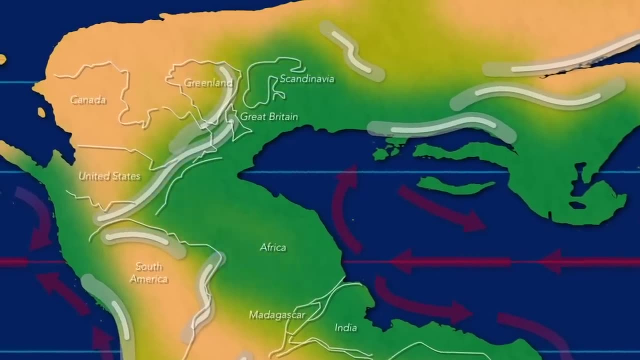 On the opposite end of this, as I mentioned before as well, a seasonal monsoon would have come into these lands, sending moisture further inland, Likely pushing the forests at the equator deeper into the continent. The forests would likely extend all the way to the central Pangean mountains, but no further. 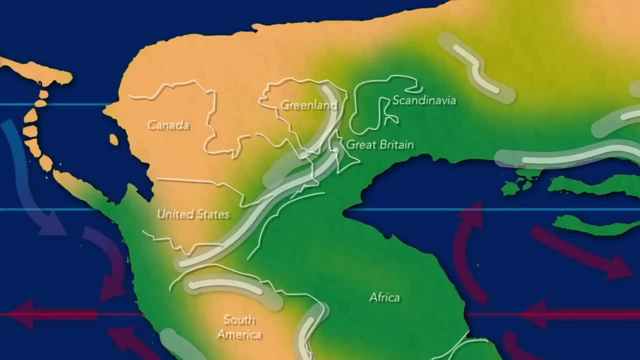 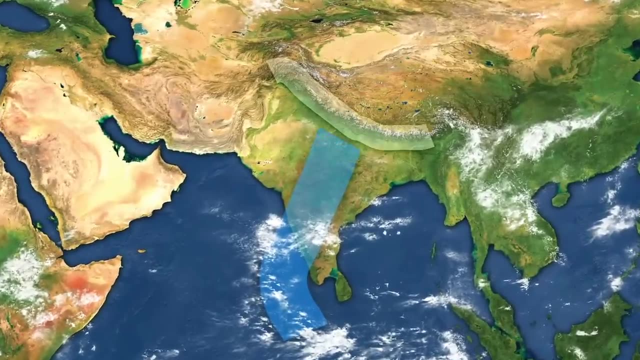 making one side of the mountain range extremely wet and rainy, While the other side dry and desert Again. we see this today in places like India, where moisture is brought all the way up until the Himalayas, and the lands on the other side, like Tibet, are extremely arid. 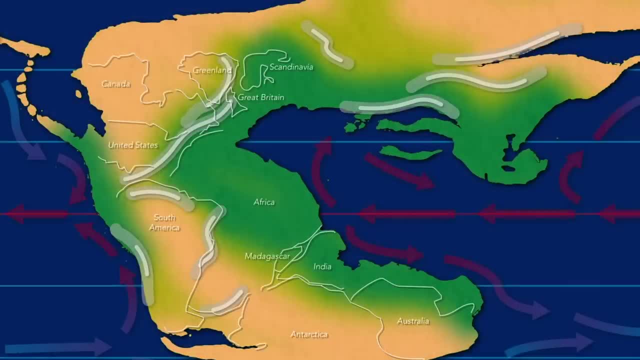 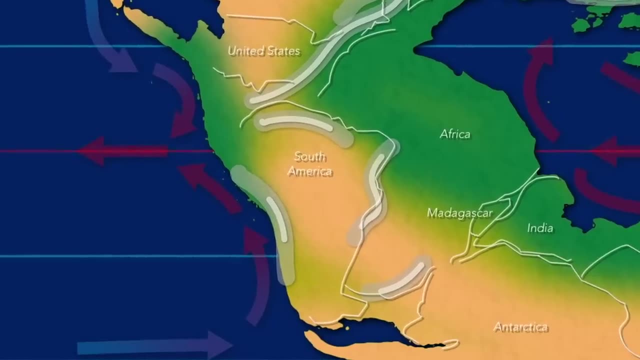 This is called the rain shadow effect. So the equatorial forest would likely not have crossed over the central Pangean mountains. This also would have prevented forests from moving too far into western Pangea. Lastly, I'm going to place narrow savannah regions around the edges of the land as the